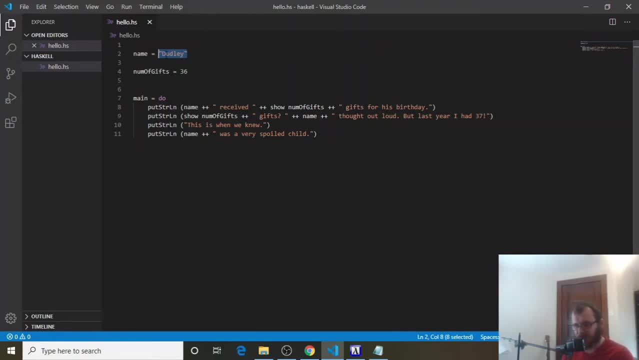 see here that name is in double quotes And it's: it's Dudley, right? So Dudley in double quotes is what's called a string in Haskell, And we can say, we can specifically say: Hey, name is going to be a string, and then we can assign Dudley to name. Now you don't have to, but we can do that. So we can say name And when to assign a type to name, we're going to use these colons and we're going to use two of them And we're going to say it's a string. So 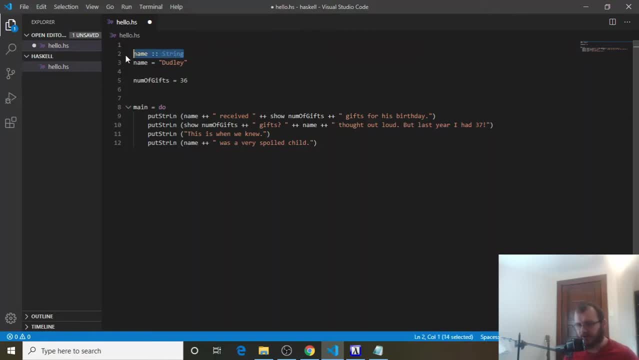 Name is a string and then underneath this we say this string is Dudley and we assign it to name. So this part up here is the type assignment. So we're going to say, hey, name's going to be a string and then we say we store Dudley. 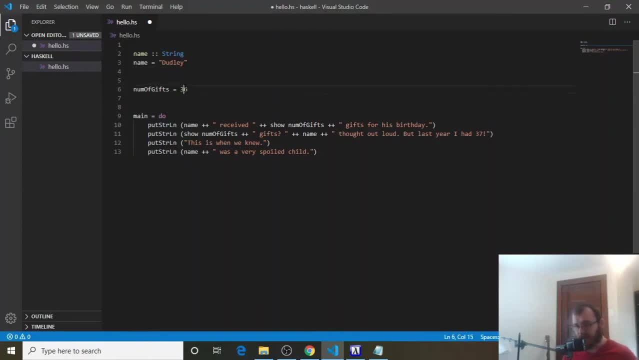 inside of name. Now 36 is a number right, But Haskell doesn't have a number type. There's a type that can replace 36, called an integer. So integers are like counting numbers: 1,, 2,, 3,, 4,, 5,, 6, 0, negative 1.. 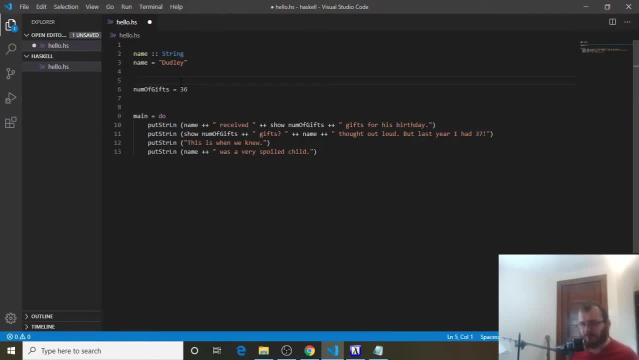 It also includes negative numbers. So any positive or negative numbers that are not decimals are called integers And we're going to use int for short as our type that we need to know. for now. There's two types: int and integer. We're just going to use int. 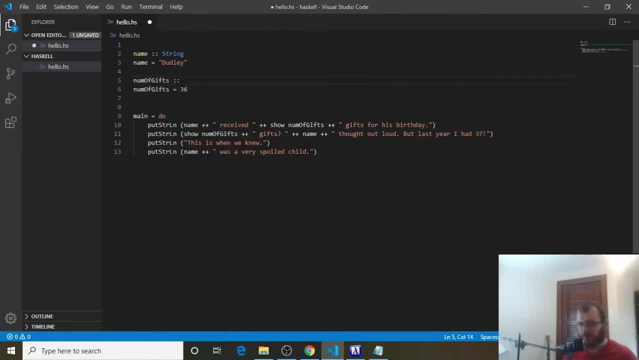 So we can say num of gifts, colon, colon, and we know number of gifts is going to be an int, so we type int And types always begin with capitals In Haskell, so capital S, capital I, And this won't make any difference when we run it. 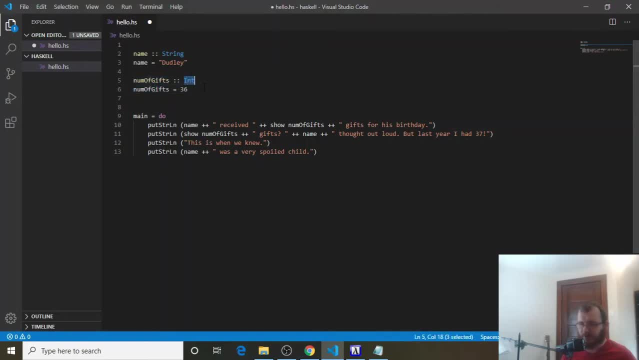 We just know hey number of gifts is an int. We're declaring it up here And we then say 36 is stored inside number of gifts. Same thing here: Dudley is a string and Dudley's stored inside of name. So this is how we specifically declare types in Haskell. 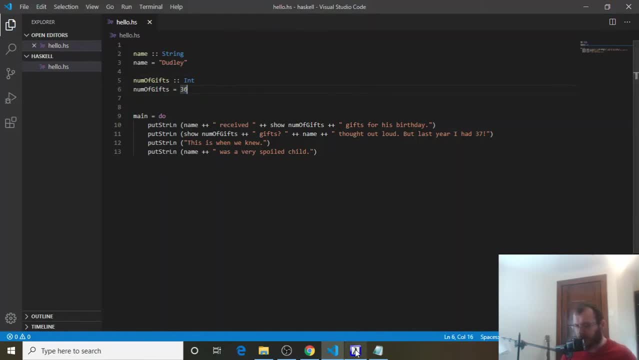 If we save that control S and run it over here, reload, evaluate, It'll still work right. We just specifically said what the types will be. Now, again, we didn't have to say these, Haskell will know. 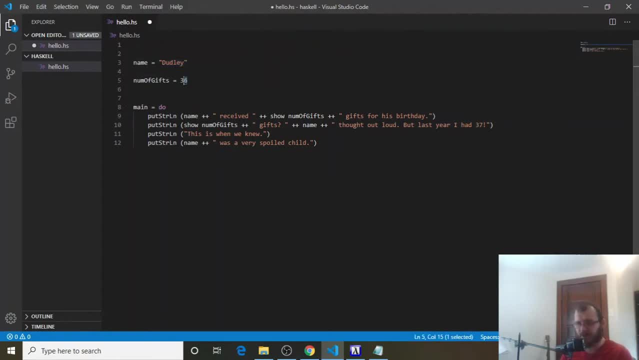 Haskell already knows that Dudley's a string. It's smart enough to know that, And it's smart enough to know that 36 is an int. But for this particular lesson, it's good to know how we declare these types above name and number of gifts. 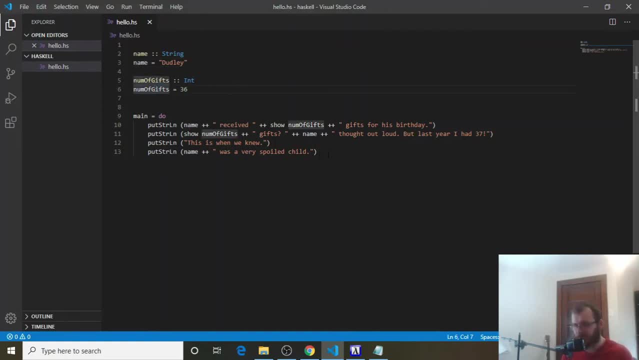 Now there's two more data types we need to talk about. So what we're actually going to do is we're going to delete this, We're going to delete this underneath main And we're just going to print these out first. So let's do. put string ln. 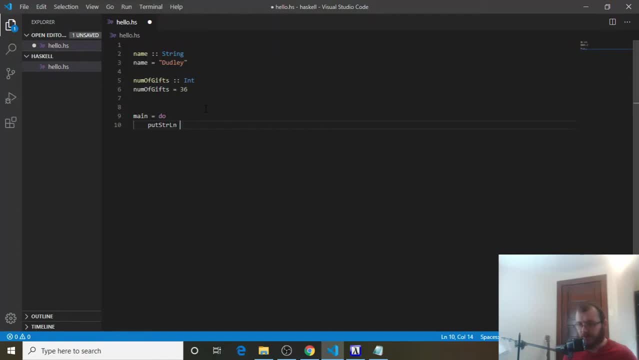 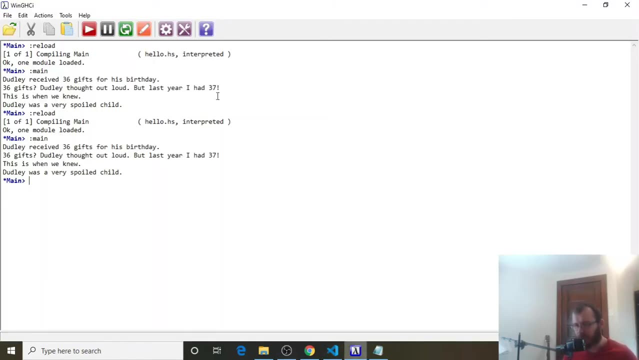 And we're going to print out the name. Now there's two ways we can do: put string ln right. We can do quotes and say name And that'll work right. If we save it, go over here, reload and run it. it'll come out Dudley. 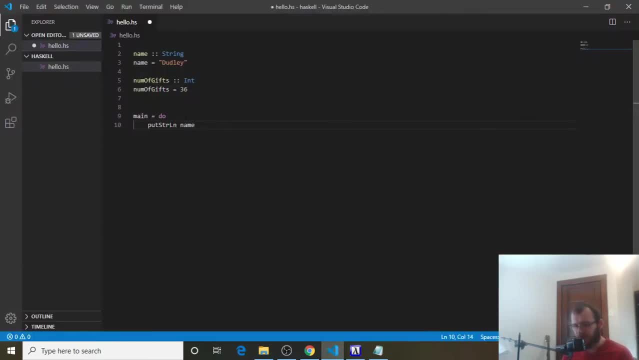 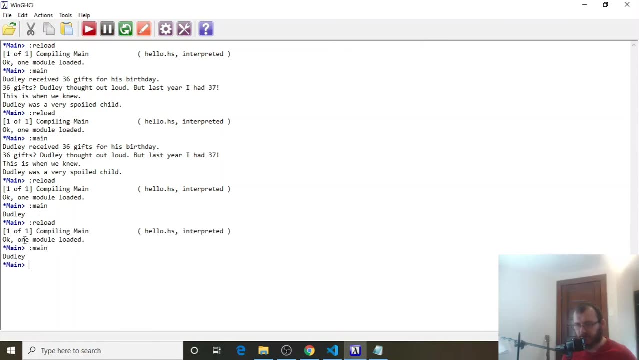 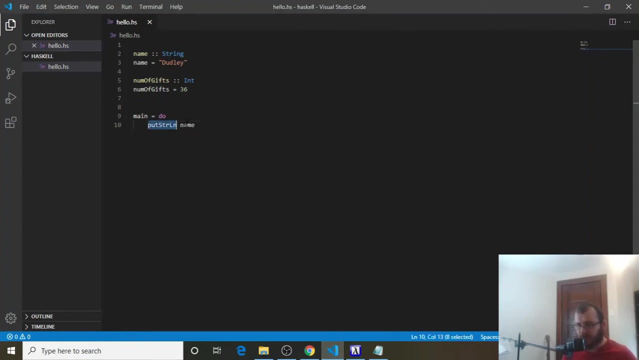 Or we can use it without the parentheses and save it, And it'll still work. It'll still print Print name: Refresh And Dudley still appears right. I'm going to clear this. So: put string ln. Anything inside of these double quotes works with. put string ln. 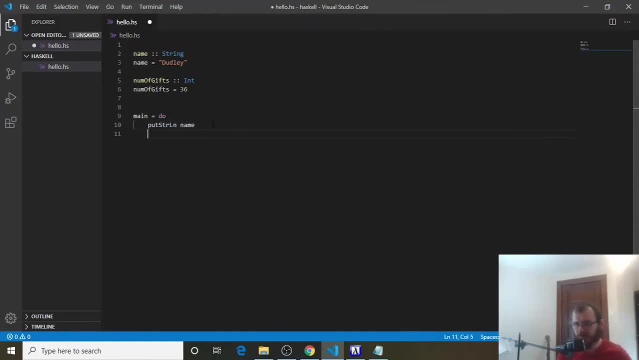 Now, anything that's not in double quotes, anything that's not a string we need to print. So let's do print num of gifts And that'll print 36 for us. Remember, main runs from top to bottom, So we put Dudley first. 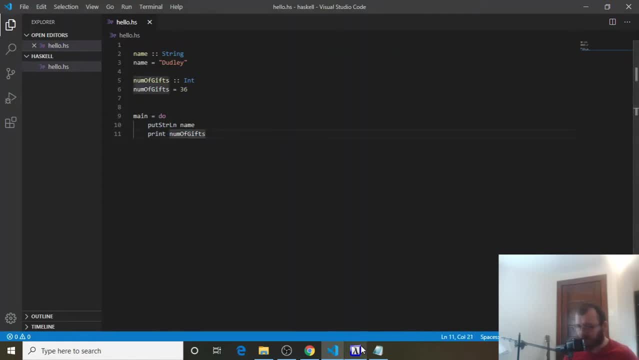 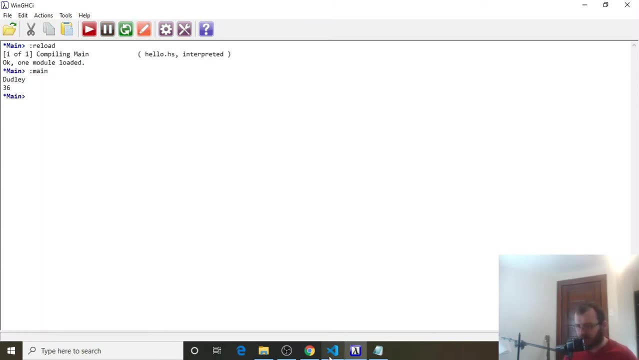 And then we print number of gifts: 36.. Save it And let's go over to the WinGHCI Refresh, Run it, Dudley 36. Perfect. So the last two types we need to talk about are char and float. 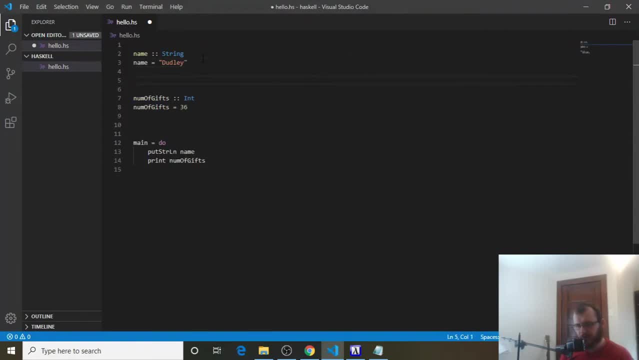 Let's start with the char type. So below name here I'm going to make a new variable And I'm going to call it my letter And I'm going to set my letter equal to in single quotes. this time, anything that's a char has to be in single quotes. 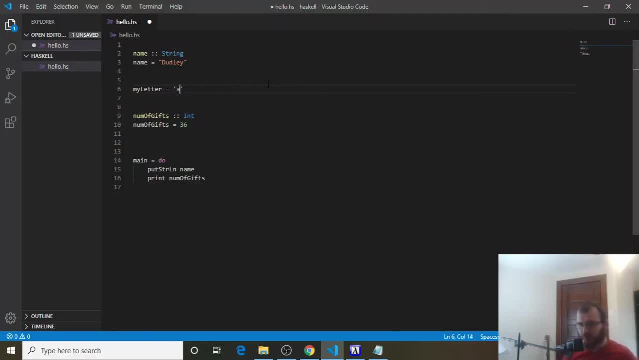 And it's only one letter. A char is one letter, So it could be A, B, C, Z, capital A, capital Z, capital B, anything like that, right? So as long as it's one letter, that's a char. 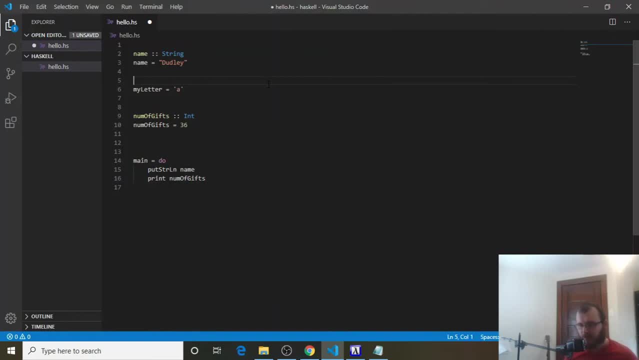 So let's set it equal to A for now, And above that, to declare the char type right, we can say: my letter colon, colon and it's char, And char is short for character. So a character is just one letter. 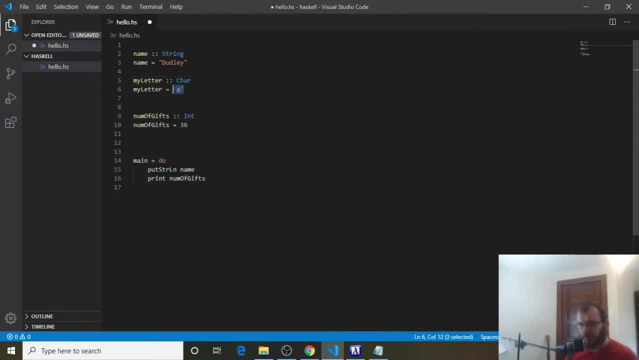 My letter char And then we store the char in single quotes inside of my letter. Now remember anything, save it. anything that is a string can be used with put string LN to print it. Anything that's not a string has to use print. 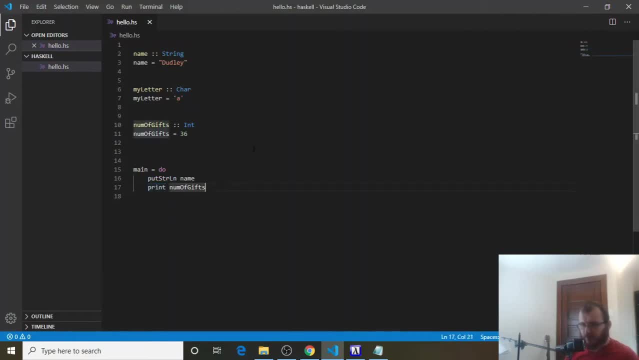 So in order to print this character, we need the print function down here And print's a function, so is put. string LN is a function. Again, we'll get the functions in just a bit, but you can kind of know that those are functions for now. 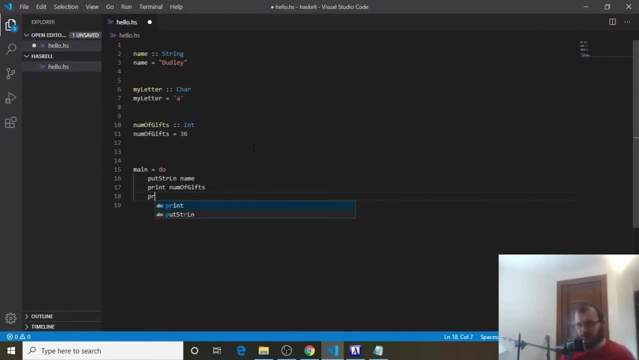 And we're giving variables to them to print to the console. So we can do print my letter underneath number of GIFs right and save it. So now this main function will know, it'll know to look for a name up here. 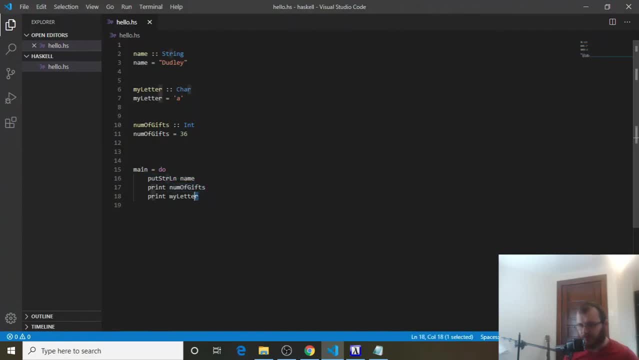 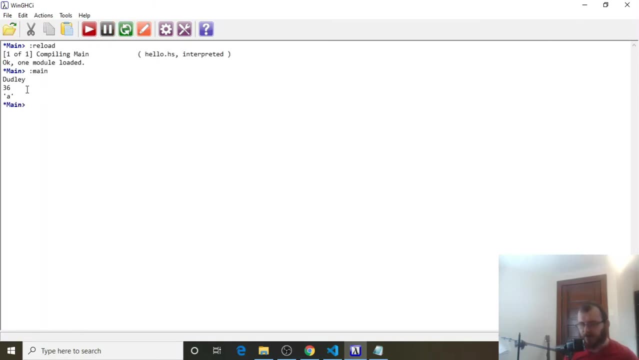 And it'll print name, then it'll print number of GIFs, then it'll print my letter. So save, go to the WinGHCI, clear it if you haven't already. reload and run it. Dudley 36A. 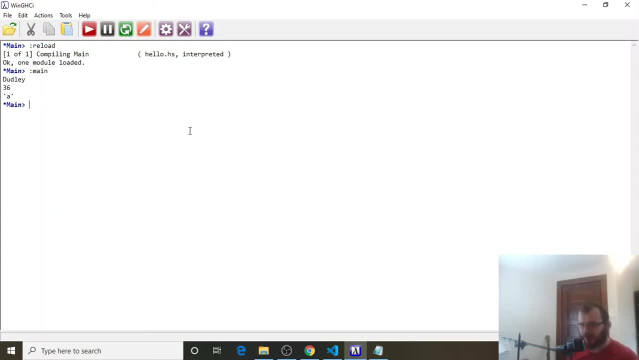 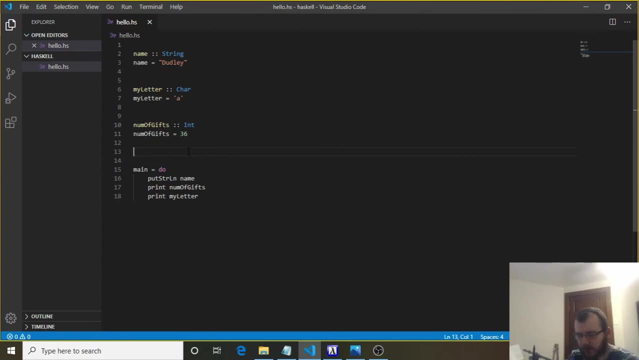 Perfect. Now let's suppose the last thing we need to talk about Is a double And the type is called a double. So back here we go, And to create a double we're going to write: let's say, Dudley has a GPA. 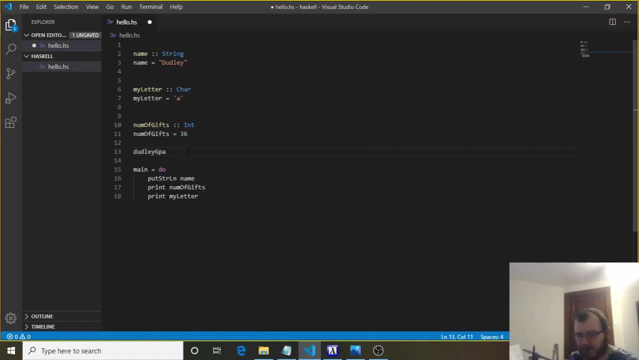 So Dudley GPA, because Dudley goes to school somewhere, right, And we're going to set that equal to the double type And a double is a decimal, So any number that's a decimal, it's going to be a double. It could also be a float, but we're just going to use double for now. 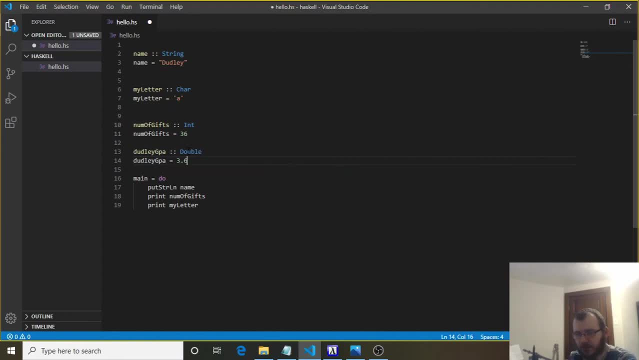 And then underneath we can say: Dudley GPA equals 3.6, because it's a decimal. And now let's go down here to main: equals do, And the last one we're going to print is Dudley GPA, So we can save it. 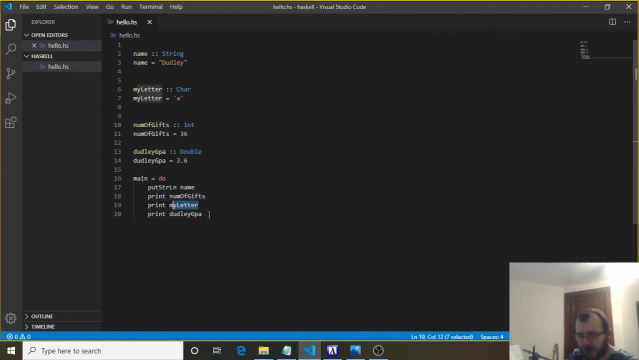 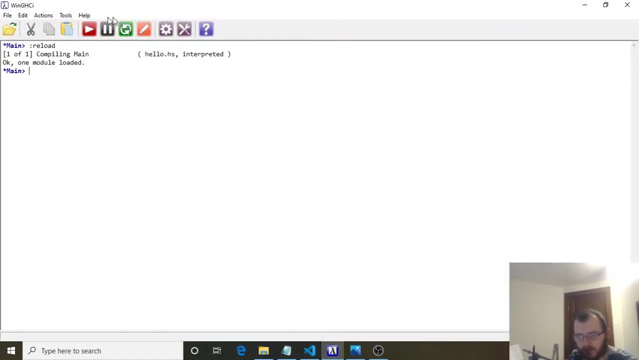 And now it'll print the name, the number of GIFs, my letter, and then it'll print Dudley's GPA. So save, go back to the WinGHCI. We're going to reload the file and evaluate it and run it. So there it is. We printed 3.6 out.